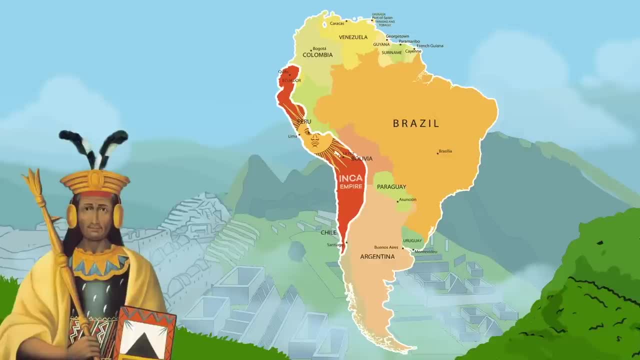 along the Pacific coast of the continent. Today, that area covers most of Peru, Ecuador, Bolivia, Chile and northwest Argentina. The Incan civilization lasted just 200 years until the Spanish invaded and captured most of the empire during the 16th century. The ancient city of Machu Picchu, which means Old Mountain, was rediscovered in 1911 and is considered one of the seven new wonders of the world. Today, South America is the fourth largest continent in the world, with an area of about 6.8 million square miles. 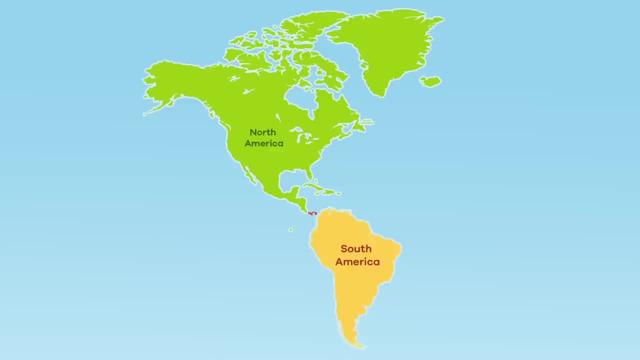 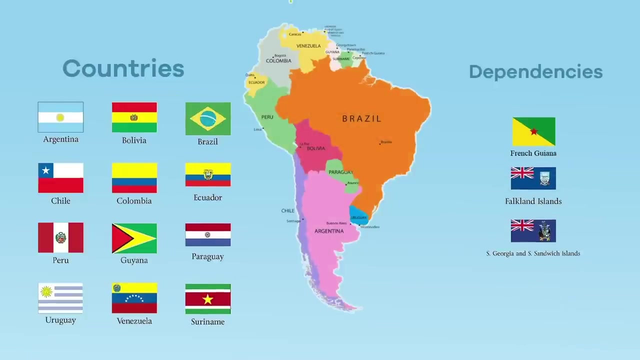 It is connected to North America via the country of Panama, Bordered by the Pacific Ocean to the west, the Atlantic Ocean to the east and the north, and the southern or Antarctic Ocean to the south. it includes 12 countries And three dependencies. 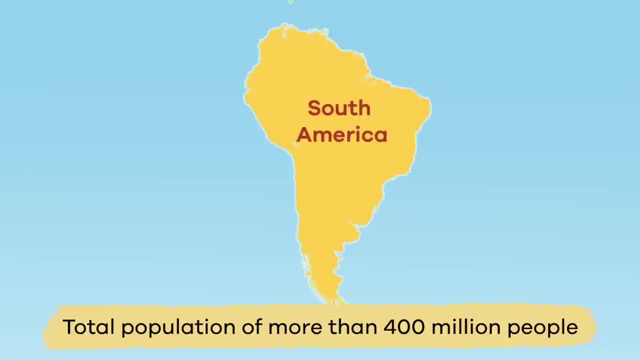 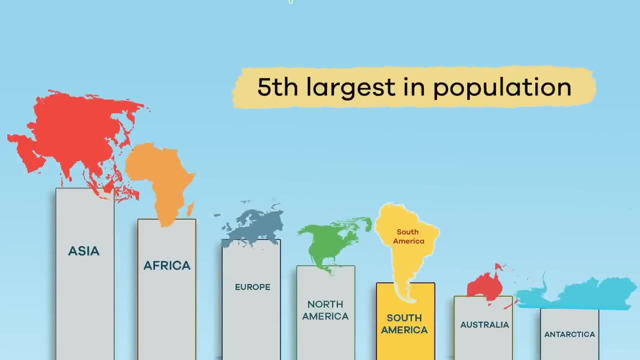 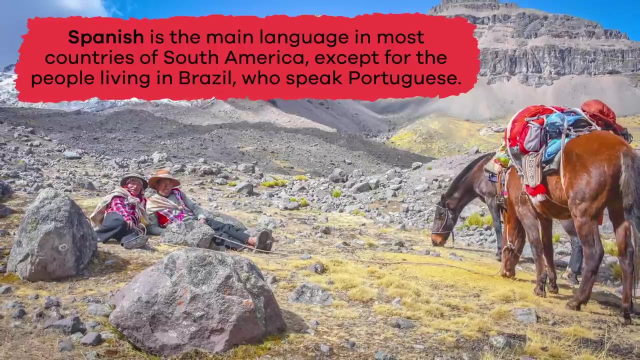 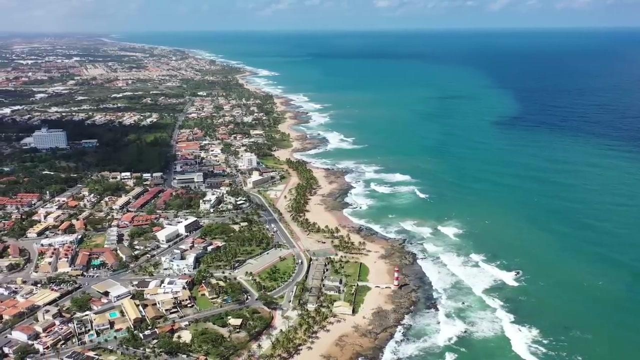 with a total population of more than 400 million people, making it the fifth largest in population of the seven continents. Spanish is the main language in most countries of South America, except for the people living in Brazil, who speak Portuguese, Many people speak English as a second language. 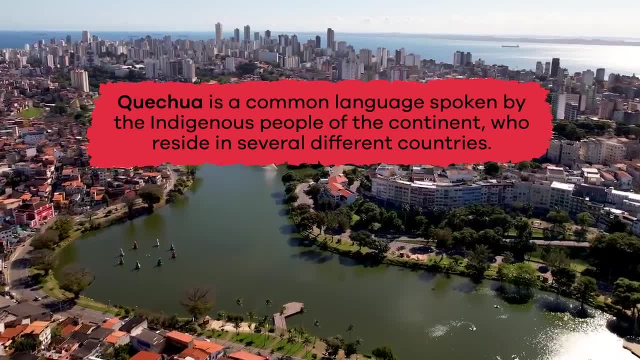 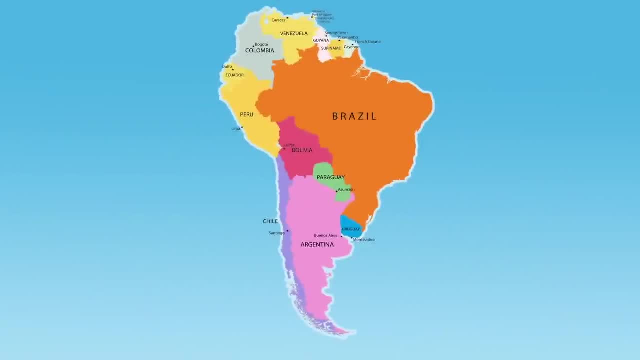 Quechua is a common language spoken by the indigenous people of the continent who reside in several different countries. Here is an interesting fact: There are only two landlocked countries inside South America: Bolivia and Paraguay. All of the other countries in the continent are partly bordered by the ocean. 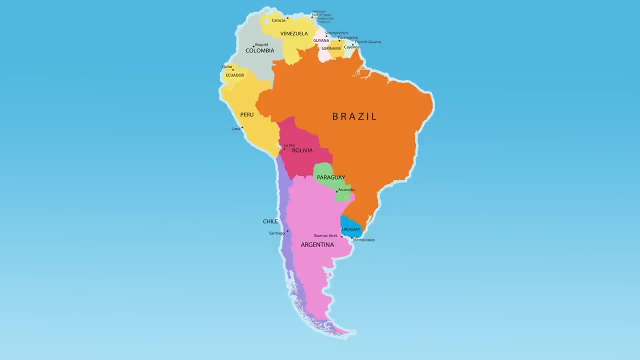 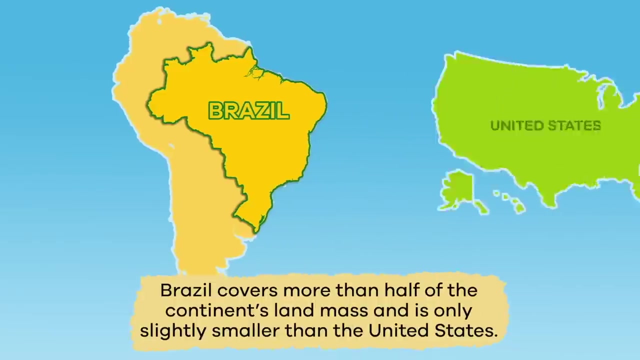 Take a look at this map of South America. Can you guess which country is the largest? If you said Brazil, you are correct. Here is an interesting fact: Brazil covers more than half of the continent's landmass and is only slightly smaller than the United States. 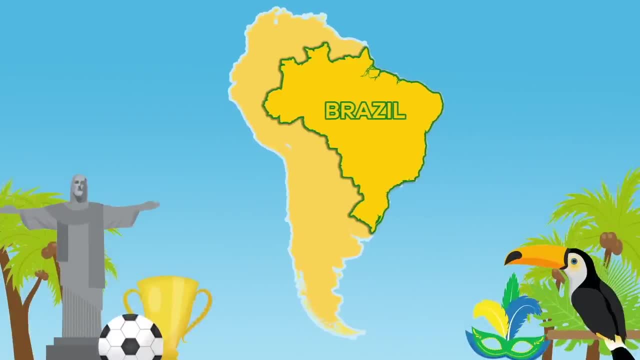 Brazil is the fifth largest country in the world in size and population. Brasilia is the capital city of the country. Sao Paulo is the most populous city in Brazil and in South America as a whole, with a population of nearly 15 million people. 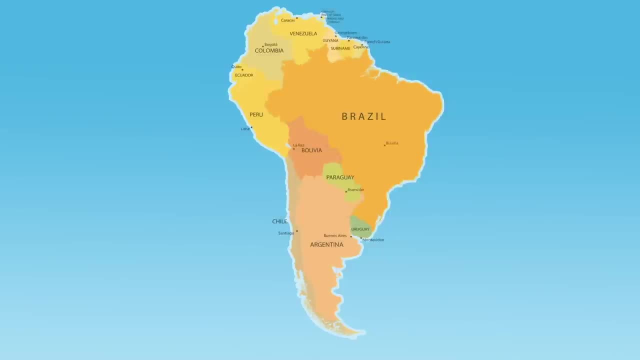 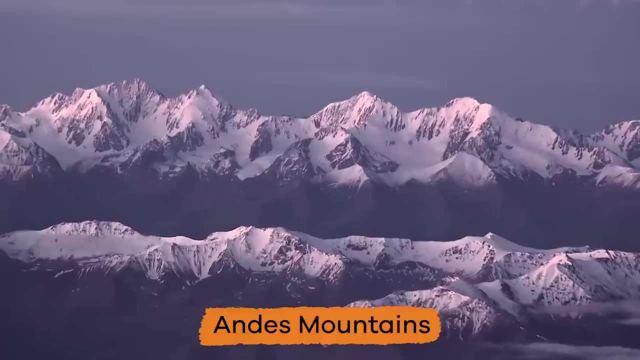 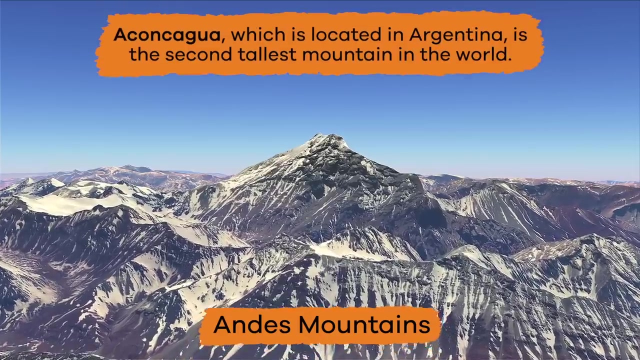 Other South American countries include Argentina, Bolivia, Suriname and Chile, and many more. Remember how we mentioned that the Incan tribe lived by the Andes Mountains. The Andes are the longest continental mountain range in the world And its highest mountain, Aconcagua, which is located in Argentina. 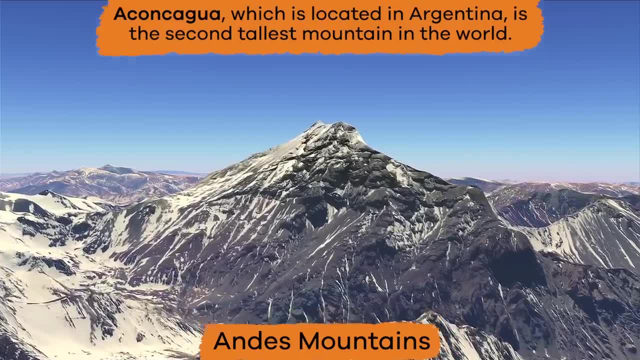 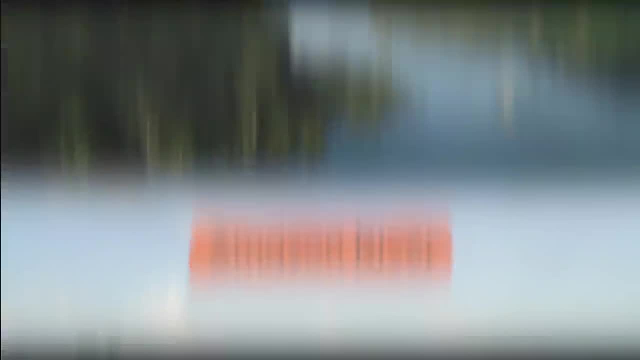 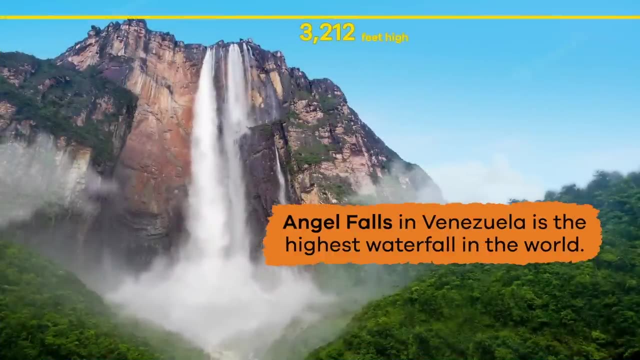 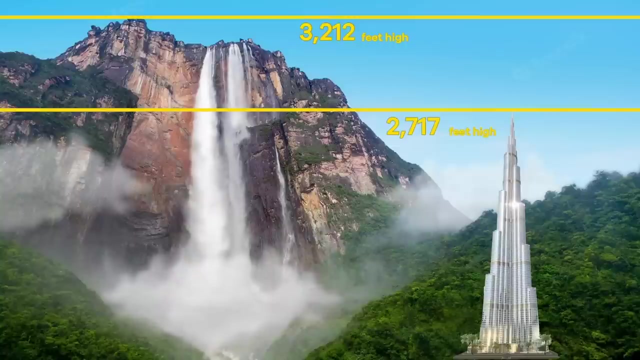 is the second tallest mountain in the world. One of the longest rivers in the world. the Amazon is also in South America At 3,212 feet high. Angel Falls in Venezuela is the highest waterfall in the world That is around 500 feet taller than the Burj Khalifa. 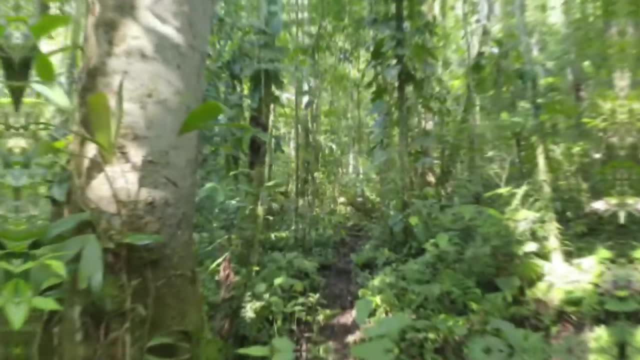 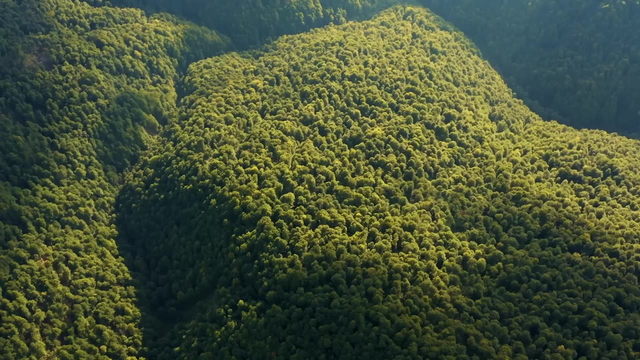 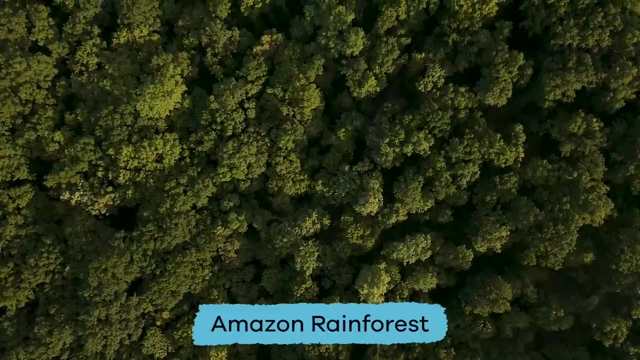 which is the tallest building in the world. South America's climate is mostly tropical, with grasslands, savannas and the largest rainforest in the world, the Amazon Rainforest. Because of the Amazon Rainforest, South America has lots of valuable trees. 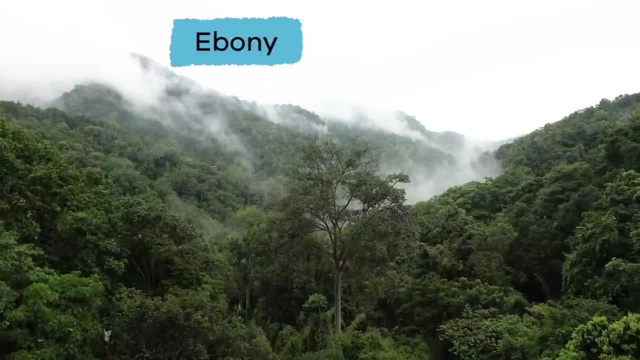 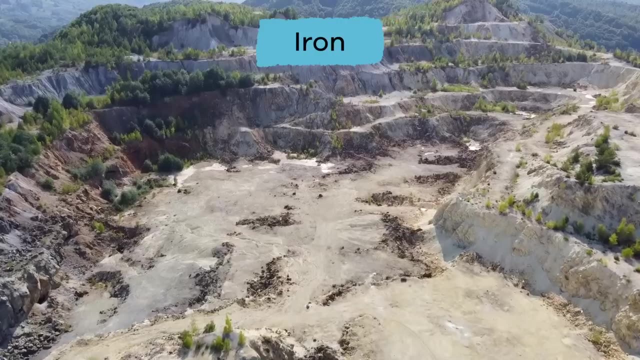 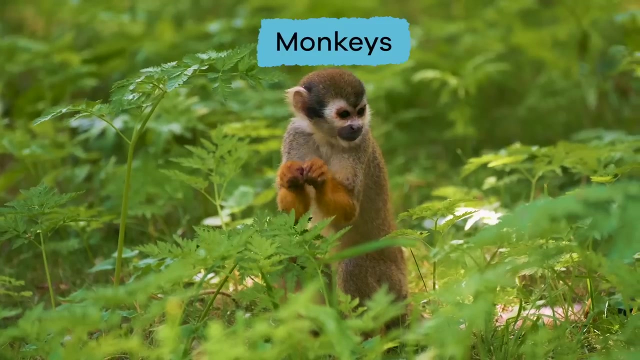 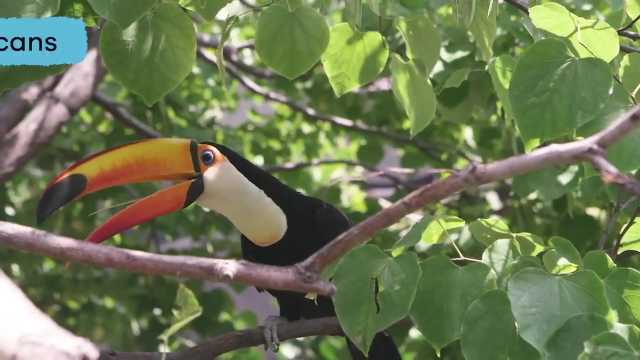 such as mahogany, ebony and rubber, plus many natural resources like oil, iron, gold and gemstones. Wildlife like jaguars, monkeys, anacondas, llamas, piranhas, toucans, cougars. 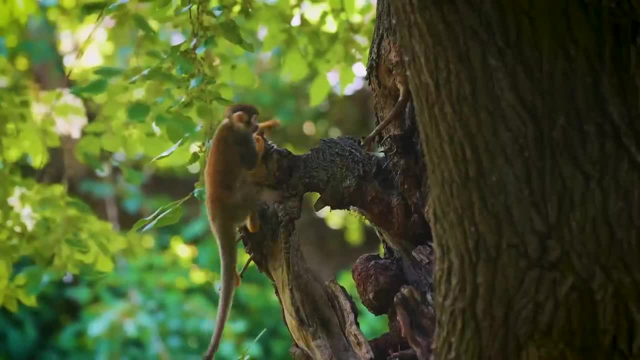 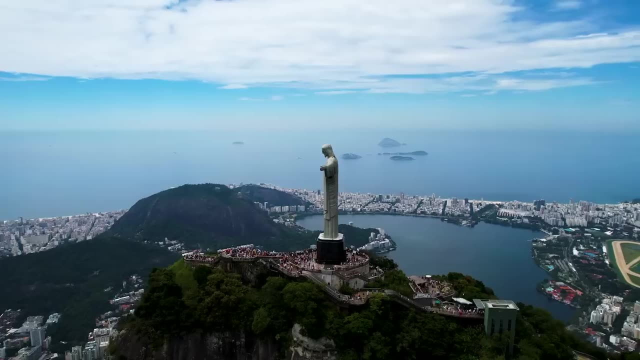 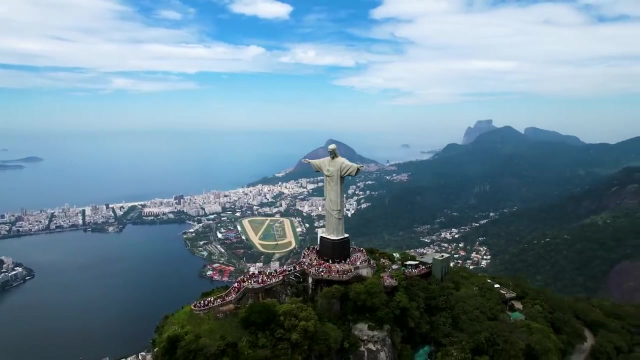 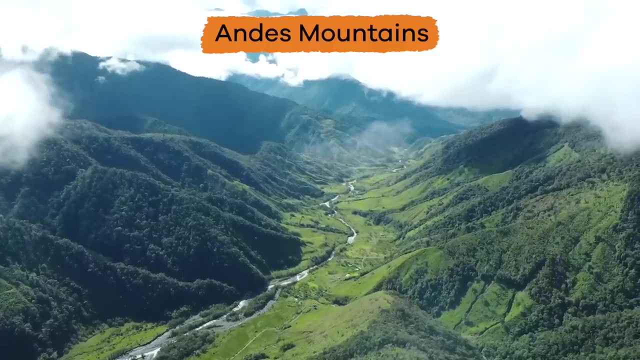 and condors all call South America their home. Along with amazing wildlife and natural resources, there are lots of exciting attractions that bring tourists from all over the world to South American countries. We have already mentioned the ancient city of Machu Picchu, the Andes Mountains, the Amazon River and Rainforest. 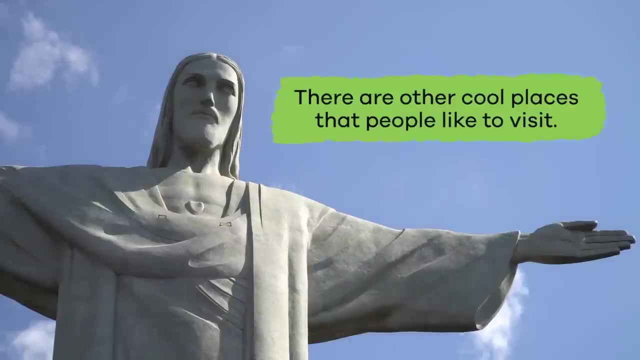 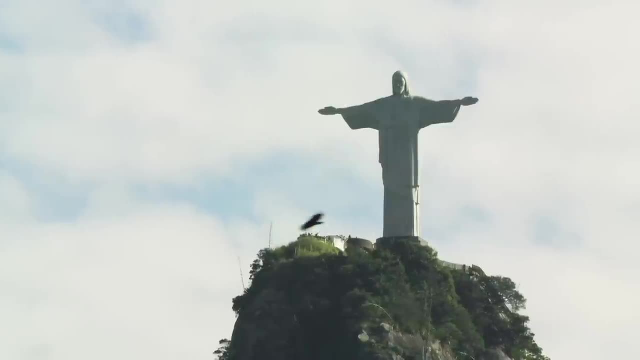 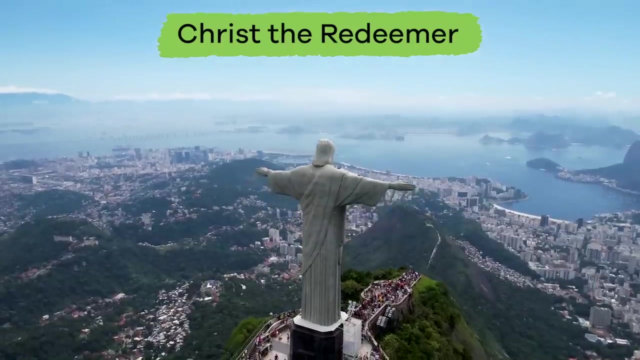 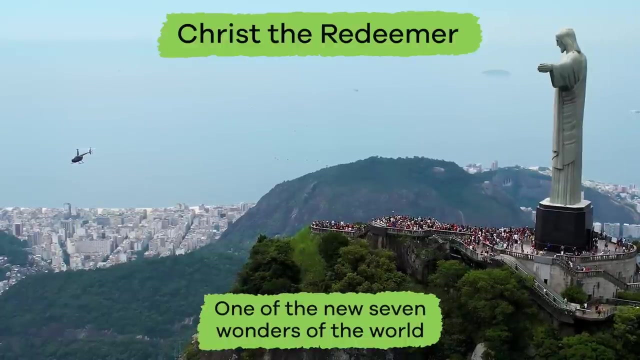 and Angel Falls. But there are other cool places that people like to visit. In Brazil there is a huge 125-foot-tall statue that is called Christ the Redeemer, which overlooks the city of Rio de Janeiro. It is considered one of the new seven wonders of the world.